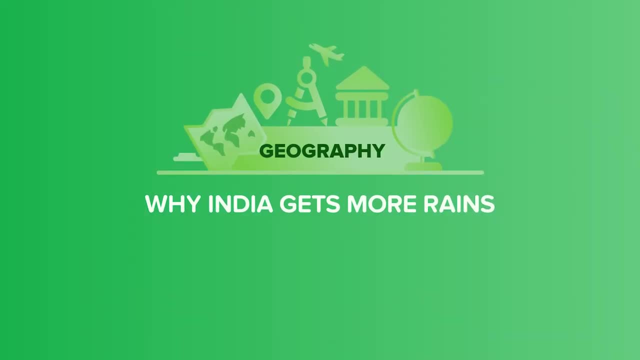 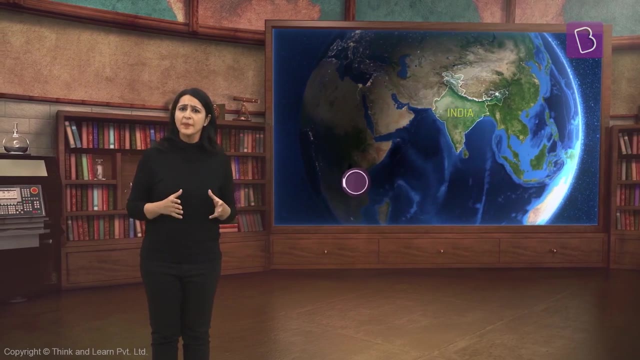 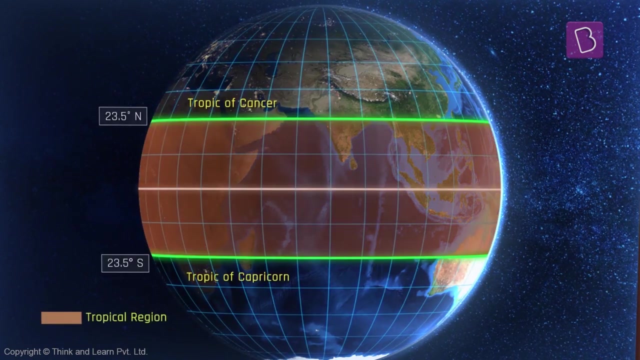 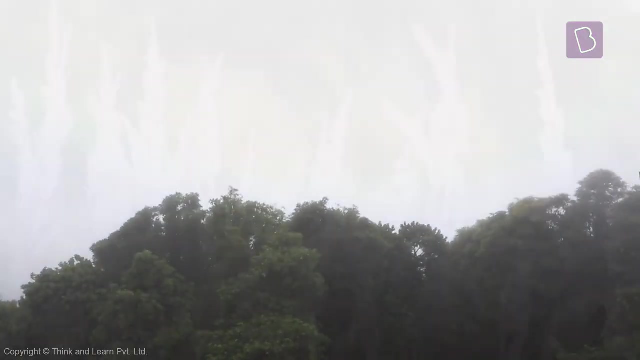 India's climate is typically called a tropical monsoon. Tropical is just a word used to describe regions between the Tropic of Cancer and the Tropic of Capricorn. And as for monsoon, the word monsoon actually comes from the Arabic word mausim, which means season. 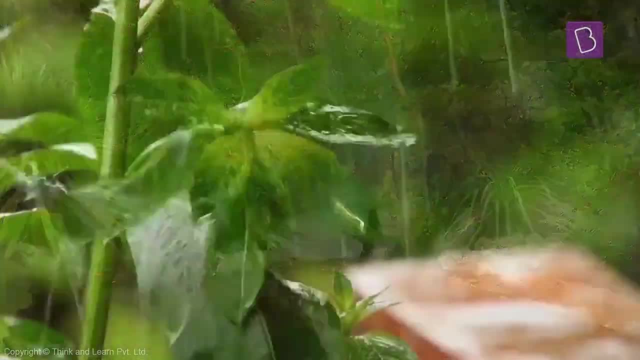 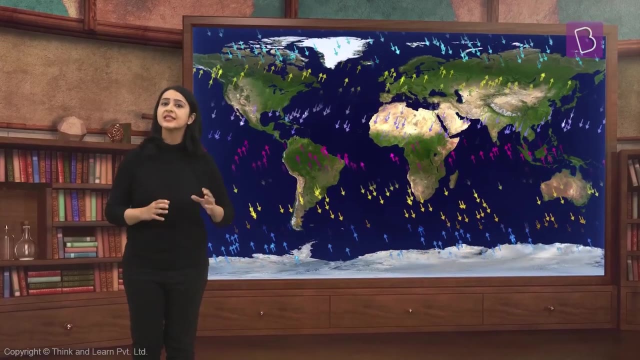 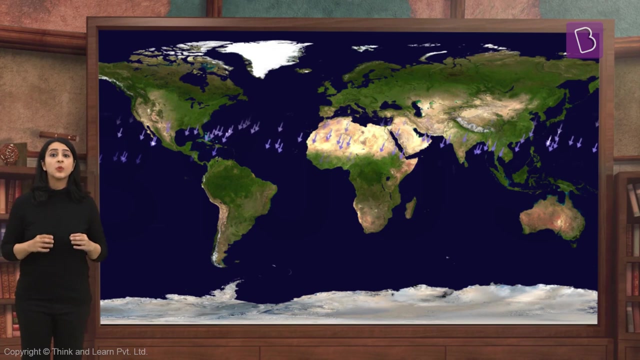 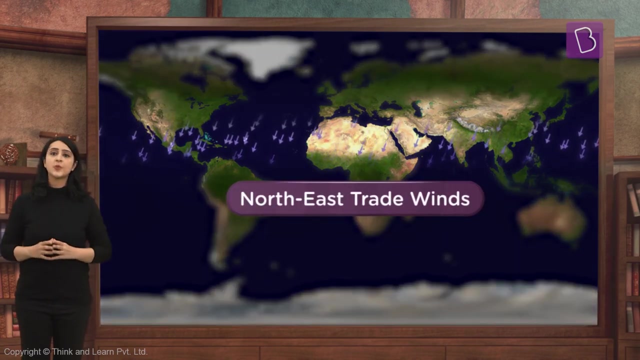 Listen, the monsoon winds are the reason that we get rains. Let me explain. Every year, heavy winds blow through the world in certain definite patterns. See those lines there. That represents the direction in which the wind is blowing, And these particular winds are called the North East Trade Winds. 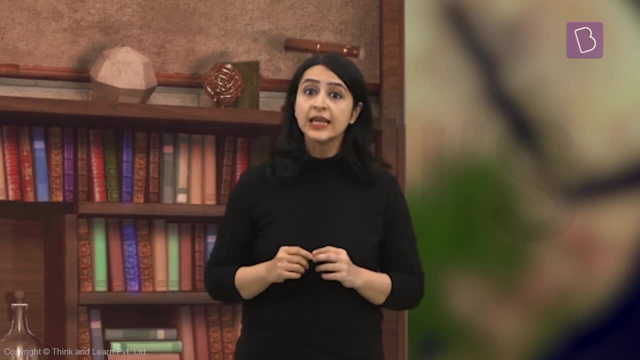 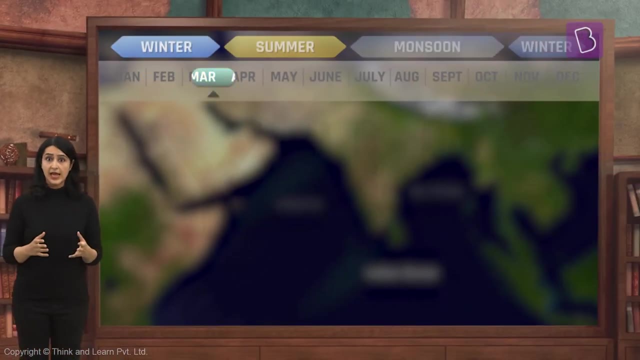 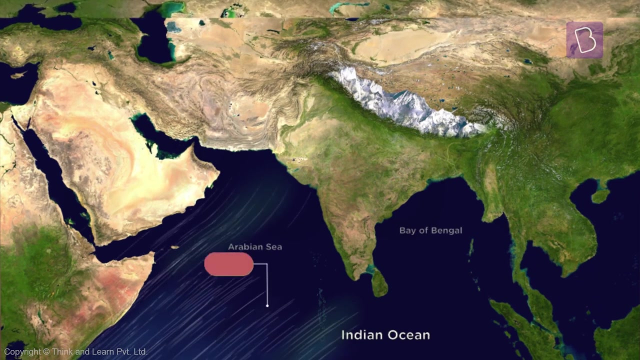 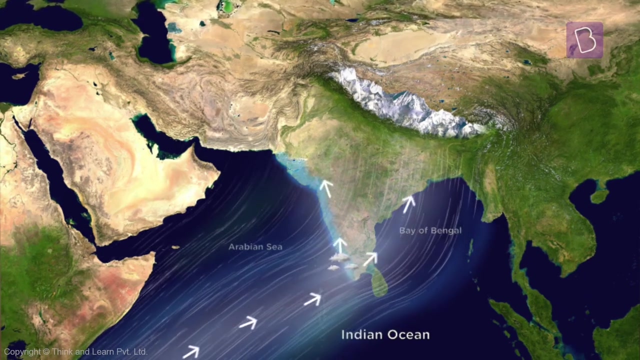 This is how the year starts. As the year keeps progressing, you go through winter first, that is, January to March, and then summer, April to June. By this time, a new set of winds from the Indian Ocean called the Southwest Winds slowly picks up the water from the oceans and brings clouds heavy with rain onto the country. 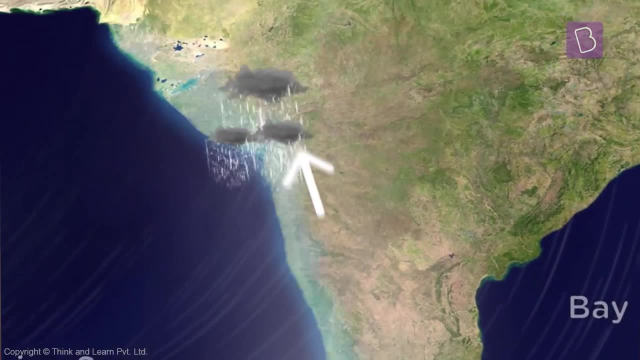 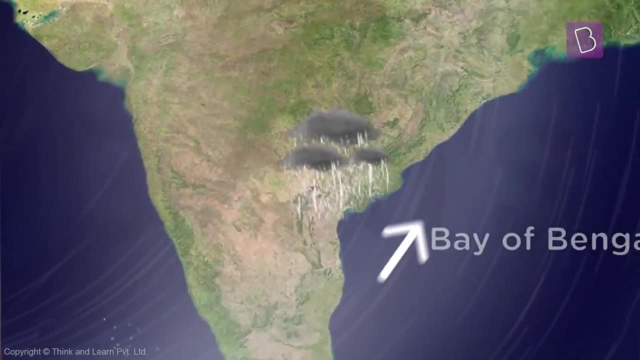 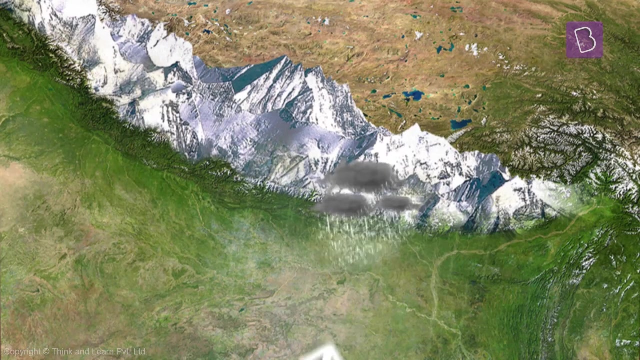 And as it gets here it goes along the western edge of the subcontinent, bringing the rain along. It also goes all the way up to the eastern side of the country and then gets deflected by the tall Himalayas. This stops the rain from going further than the Himalayas. 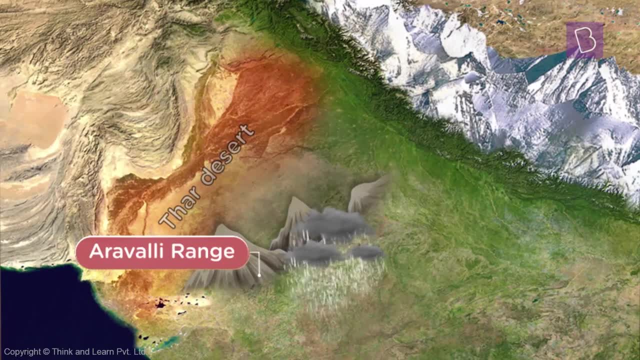 Something like this happens in Rajasthan as well. The monsoon doesn't enter this area at all. It is blocked by the Aravalli Ranges. This makes it a rain shadow area That is an area of rain, An area that the rain can't get to. 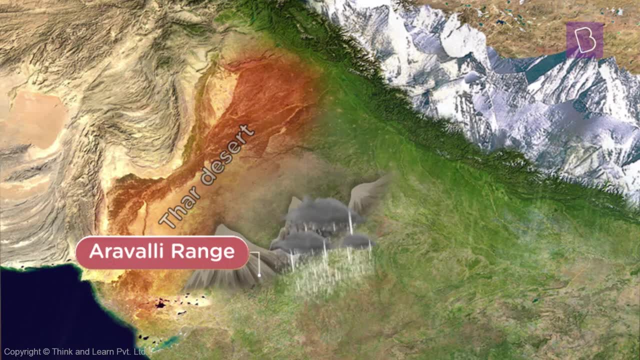 But even if the clouds could get there, there would be no point, Because by this time the clouds have already emptied all the water they brought in. That's why this part of Rajasthan is a desert. Mountains are stopping the rain, and the clouds that do manage to get over the Aravalli Ranges.